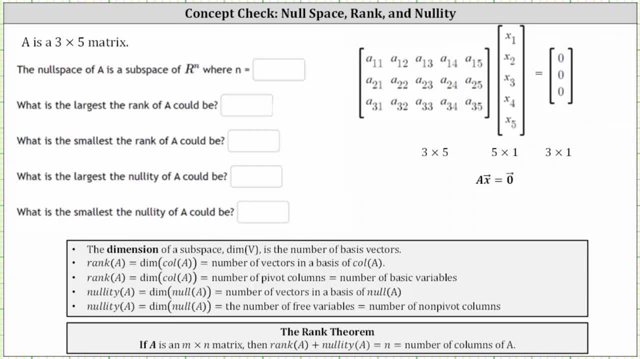 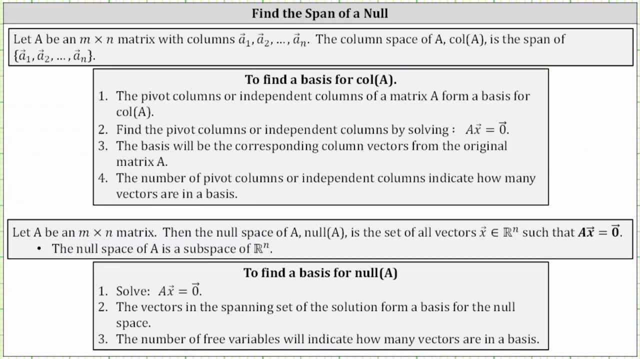 A is a three by five matrix. The null space of A is a subspace of our n where n is equal to what number? For a quick review, if A is an n by n matrix, then the null space of A is the set of all vectors x in our n. 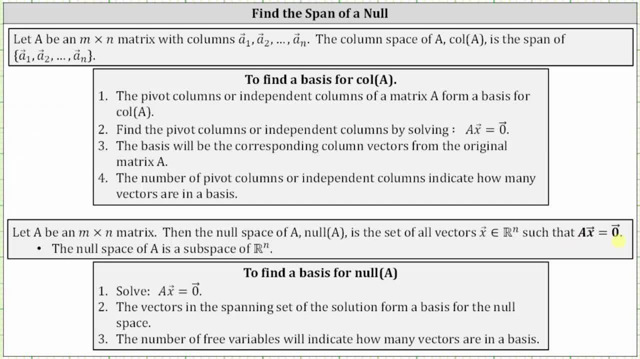 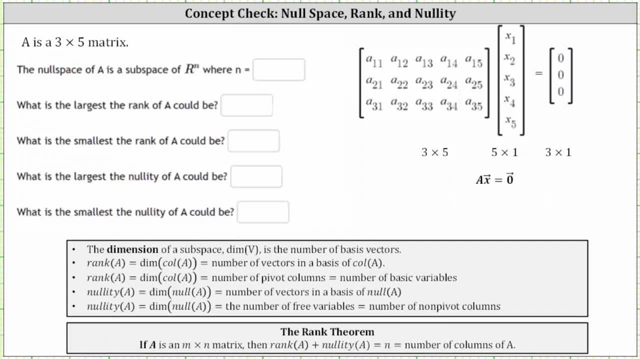 such that A times vector x equals the zero vector. The null space of A is a subspace of our n, where n is a number of columns in matrix A. So, going back to our example, because we are given a three by five matrix, 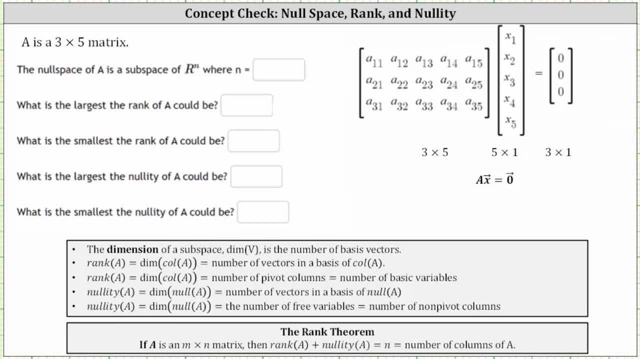 there are five columns. The null space of A is a subspace of our five and therefore n is equal to five. To better understand this, if we set up the equation A times vector x equals a zero vector. we know when multiplying matrices. 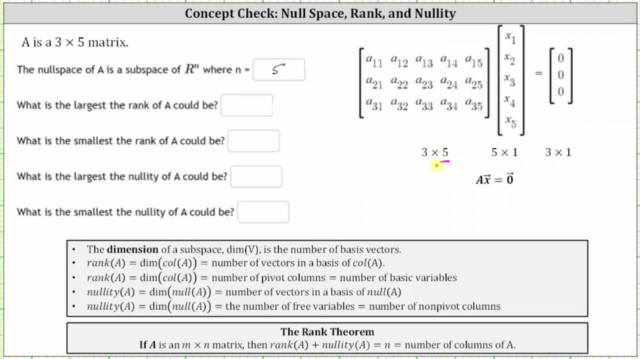 the number of columns in the first matrix must equal the number of rows in the second matrix, which indicates that vector x as a matrix must be a five by one matrix, because vector x has five components. The null space is a subspace of our five. 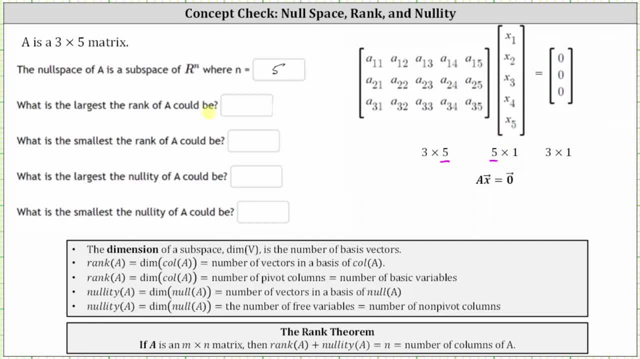 Next, what is the largest the rank of A could be? The rank of A is equal to the dimension of the column space of A, which equals the number of pivot columns. So the largest the rank of A could be would be the most number of pivot columns we can have. 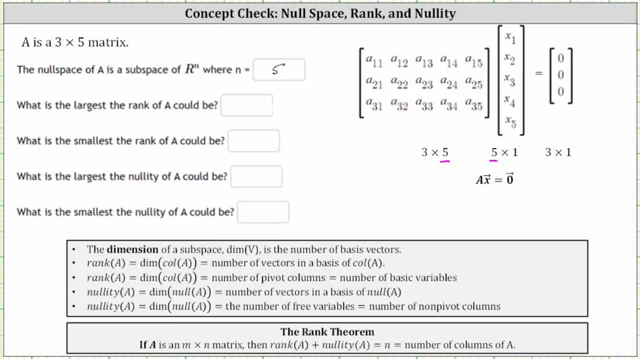 Well, we do have five columns, but they all can't be pivot columns. For example, if we had pivots in row one, column one, row two, column two, and row three, column three, we could not have any more pivots. 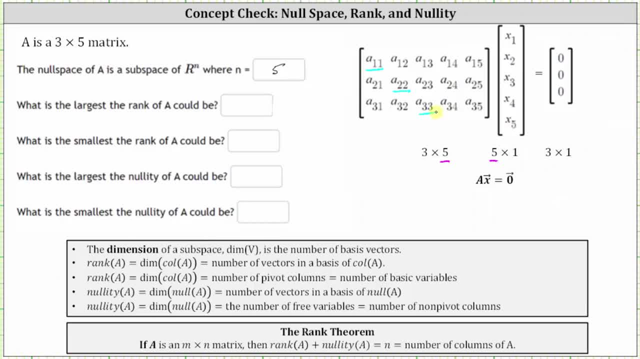 This gives us a maximum of one, two, three pivot columns. The largest the rank of A could be is three. Next, what is the smallest the rank of A could be? Well, this would be the least number of pivot columns that we can have. 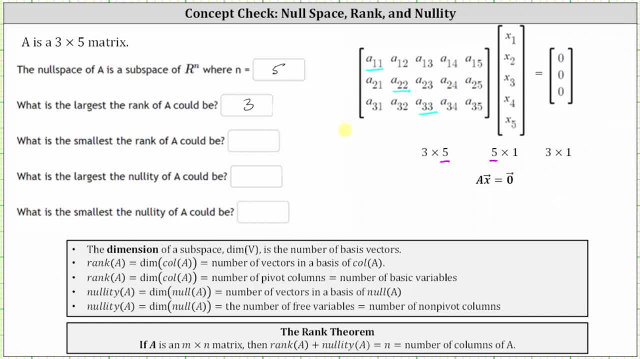 It is possible to have zero pivot columns, for example, if matrix A is a zero matrix, So the smallest the rank of A could be is zero. Before we talk about the next two questions that involve nullity, let's talk about the rank theorem. 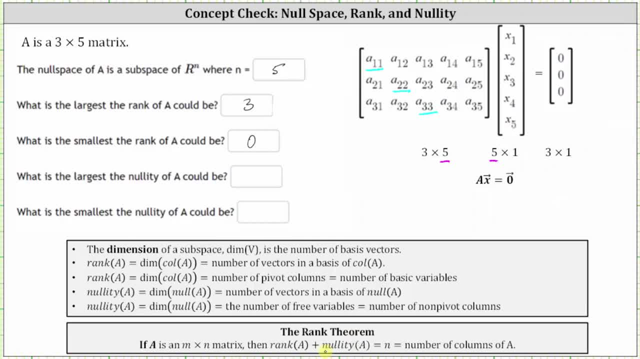 If A is an m by n matrix, then the rank of A is zero. The rank of matrix A plus the nullity of matrix A must equal n, the number of columns of matrix A. The next question asks what is the largest the nullity of A could be.